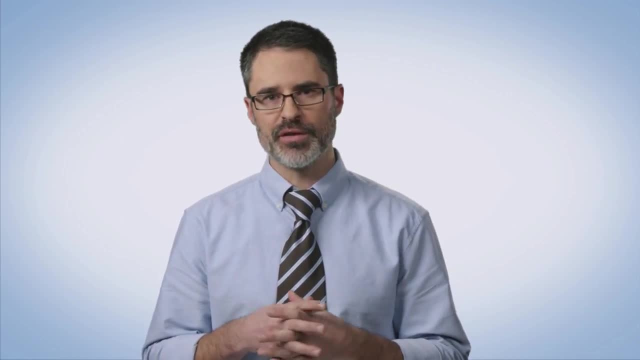 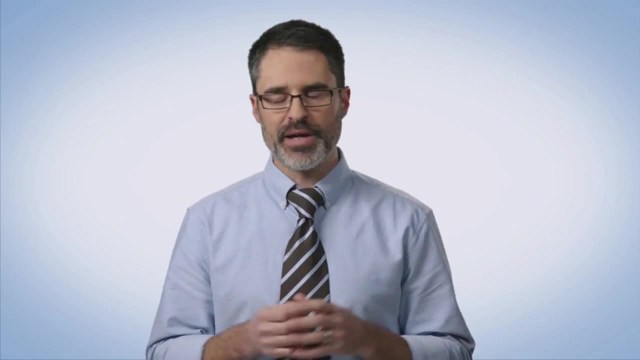 into this mess, because we really are in a mess when it comes to environmental considerations and what we need to do to get out. Many courses of this type quickly get labeled Intro to Doom 101 or Introduction to the End of the World, because much of the stuff that we're 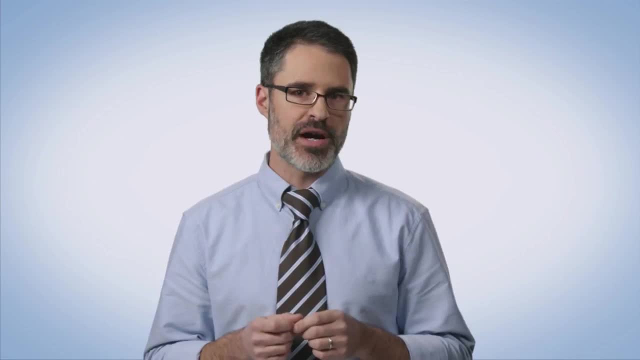 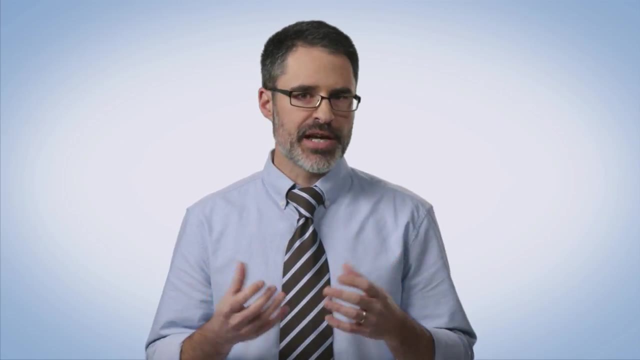 going to be dealing with is pretty dark When you start digging into the environmental situation. if you're paying attention, you'll notice that things don't look too rosy. So I teach this stuff in part because it's a great intellectual challenge. As an academic, I get jazzed up. 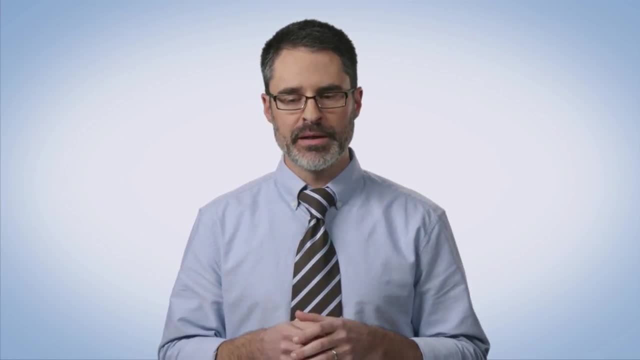 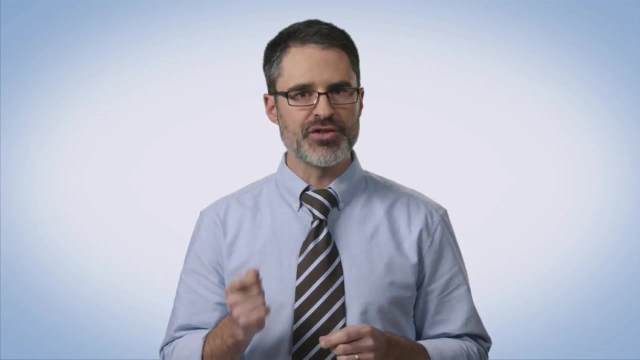 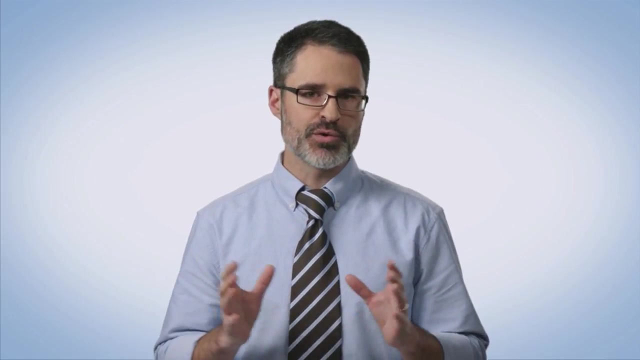 by thinking about big ideas and big questions, But I also spend time working on these issues because I firmly believe, with lots of other people, that the environmental challenge is the great challenge of our age. Every generation faces its own unique set of challenges. In the past we've had folks who have worked to 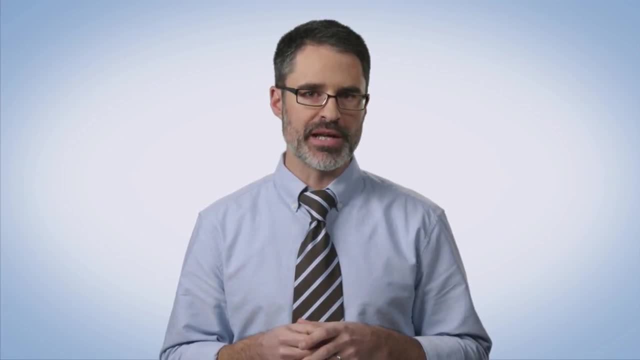 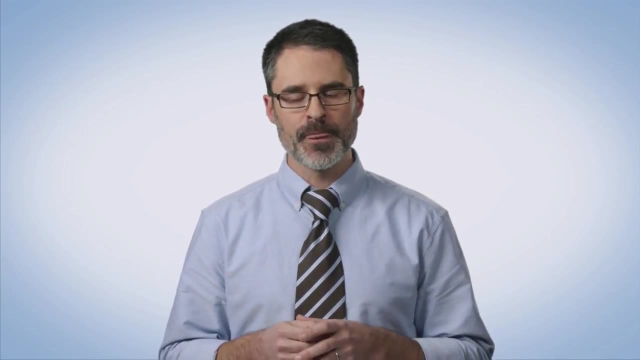 bring about greater civil rights for certain parts of the human population. We've had folks who have worked to transition us to new technological forms through the industrial revolution. We've had folks who have been in generations that have had to fight great wars and wars, and 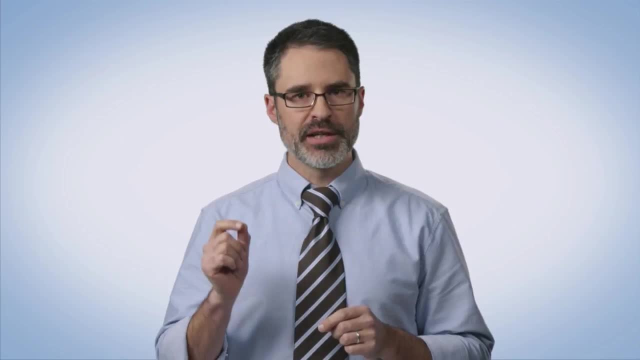 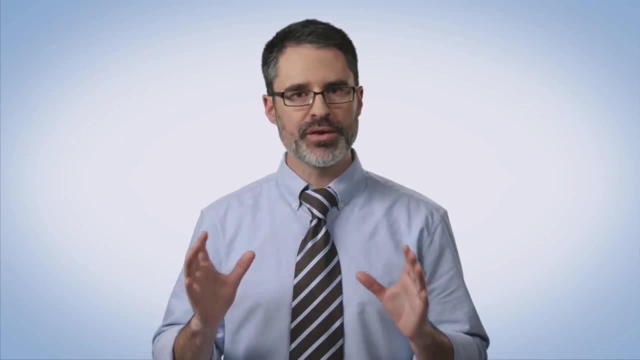 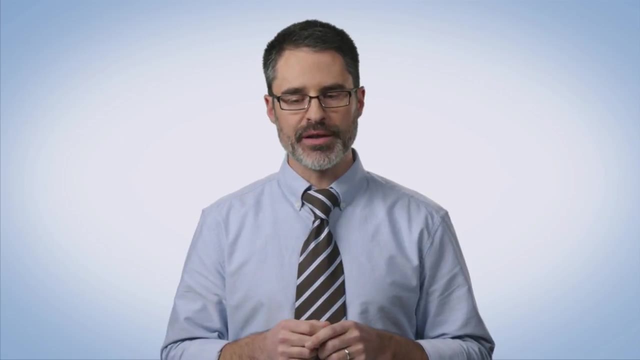 compatible with ecological realities. If we don't sort this out, nothing else matters. There's a quote from a guy I know named David Orr. David and I taught a workshop together some years ago, and during that workshop David said something that has kind of stuck with. 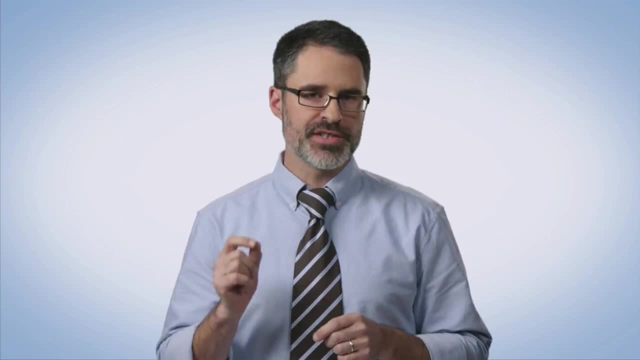 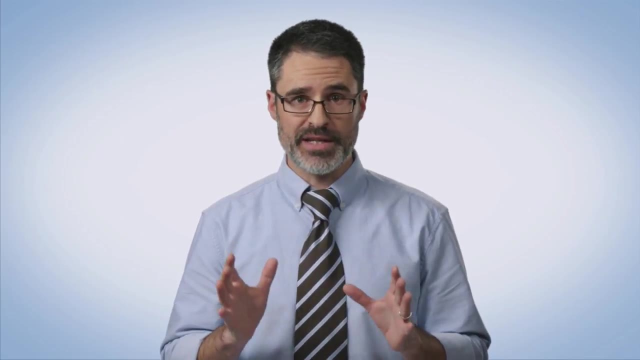 me and resonated ever since He said that if you consider the environmental situation and you're optimistic, you don't know enough, Which is pretty profound and pretty depressing. But he went on to say: if you're pessimistic then you're ineffective. 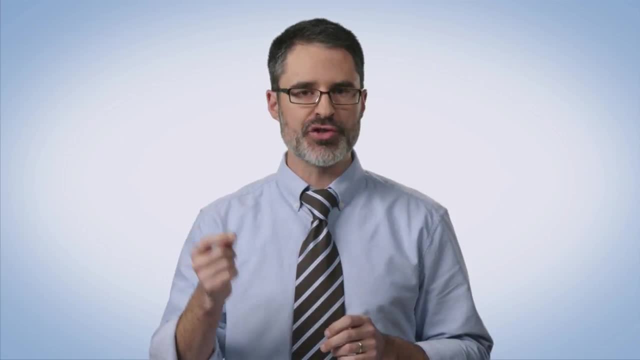 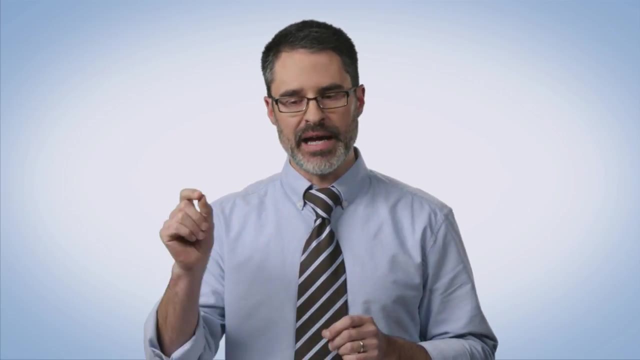 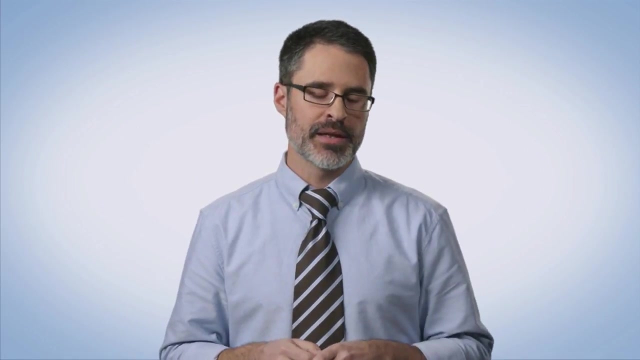 So the great challenge for us in the face of the environmental situation is to find the sweet spot between optimism and pessimism, Between being blindly optimistic and so pessimistic that we drink heavily and just kind of throw the covers over our heads. That sweet spot is hope. That's the sweet spot in the middle.